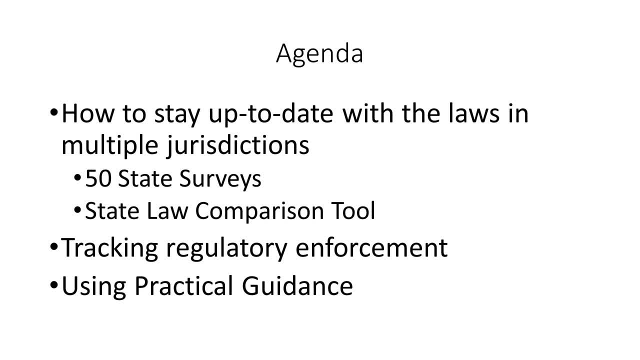 I will show you how to stay up to date on data security and privacy laws in 50 states, ensuring you are aware of regulatory trackers to follow key enforcement agencies, and I'll show you how to quickly draft and update privacy policies. I'll walk you through. 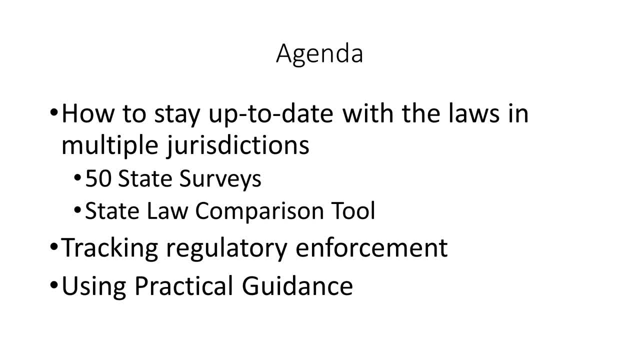 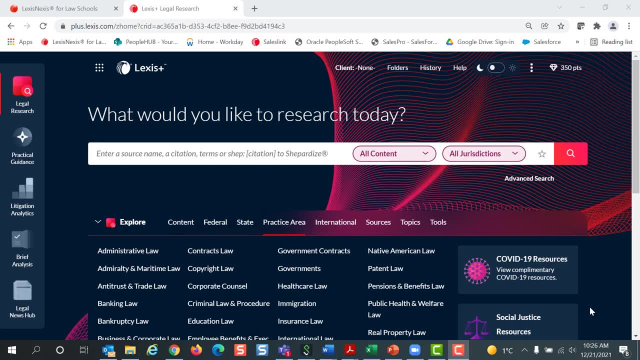 how to approach these today, and the centerpiece will be practical guidance. You're probably wondering what data security and privacy encompasses. It's a wide range of topics, including, but not limited to, cybersecurity, risk management, data breach planning and response, employment, privacy, regulatory enforcement, actions related to cybersecurity. 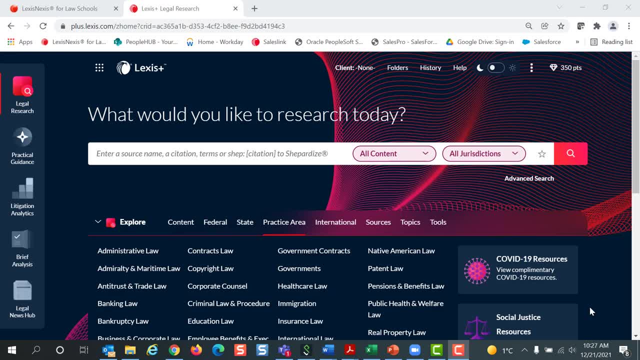 and data privacy and cybersecurity. You may also be wondering what practical guidance is and why you should use it. Practical guidance is a great tool for task-based research and you'll get practical guidance from pioneering attorneys in several areas of law, including data security and privacy, on essential skills, including compliance on all levels. 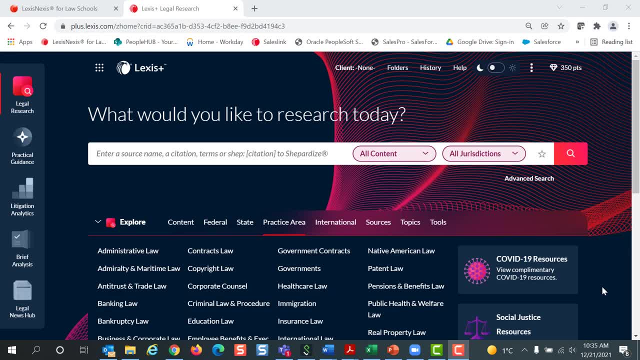 cybersecurity, risk management, how to manage data breaches, drafting policies and much more. An added bonus of using practical guidance is that we include our data security and privacy content as part of the practical guidance subscription, rather than requiring customers to buy an additional product. Now it's time to show you all these awesome and easy to use tools and resources. 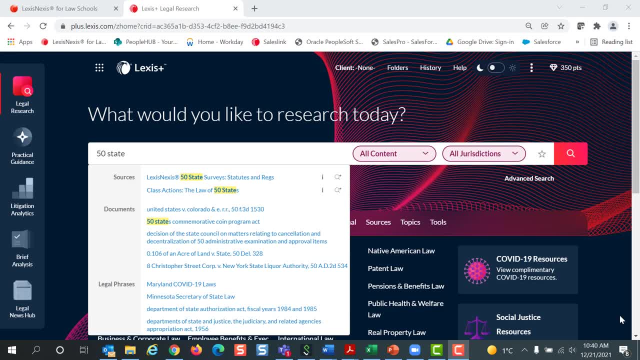 This screen is the research homepage and is where a lot of your research will begin. First, let's discuss staying up to date on laws in multiple jurisdictions. In the search box you'll see that the search wheel starts to populate relevant options. Select 50 state surveys. You'll notice that before I even complete that phrase. 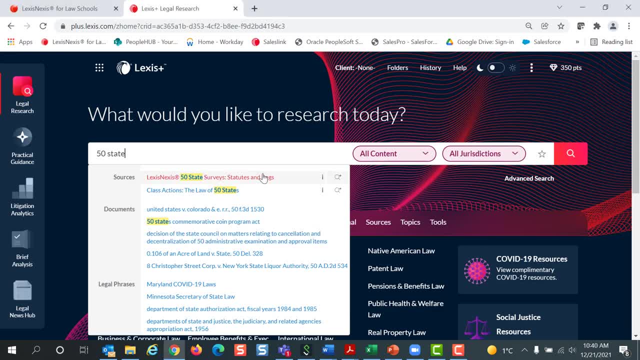 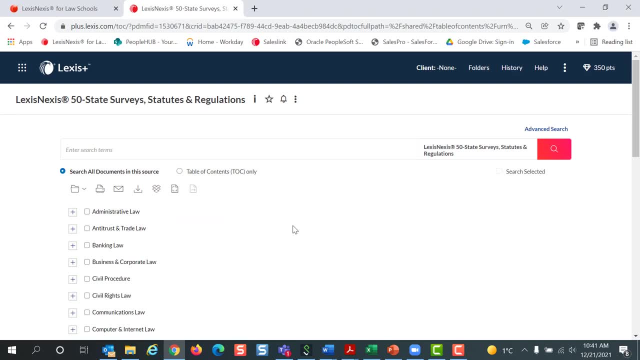 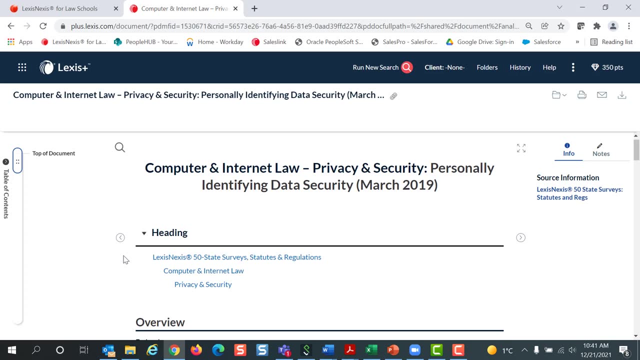 the search wheel begins to populate relevant options. Select 50 state surveys. You'll note several options here, but we'll focus on computer and internet law and, more specifically, the privacy and security option. Once you select the privacy and security section, 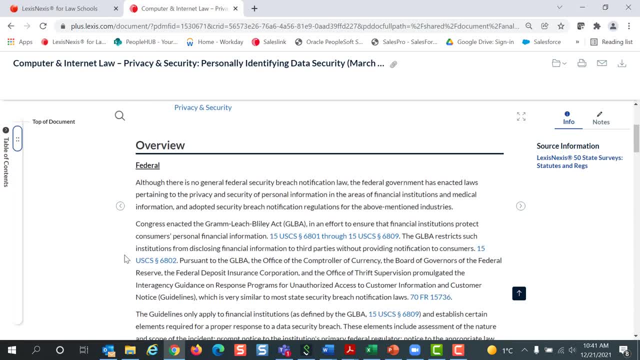 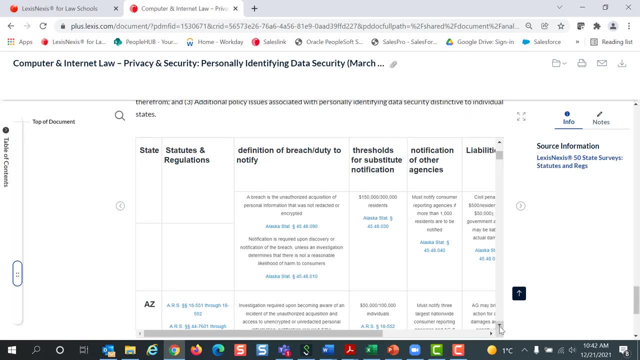 you'll see a nice overview about your topic And if you continue scrolling, you'll end up at a wonderful chart with information about this topic, broken down by jurisdiction. This will allow you to quickly compare all of those jurisdictions. Plus, there are links and citations here, so it is a huge time saver. 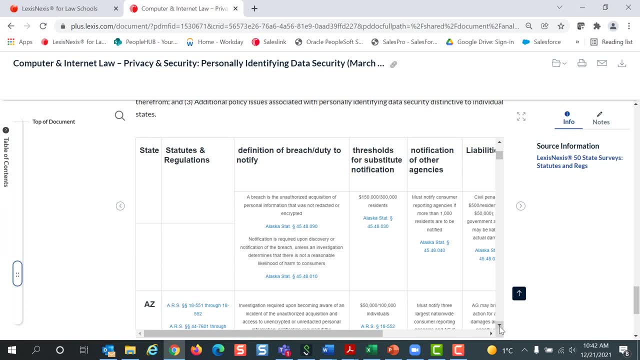 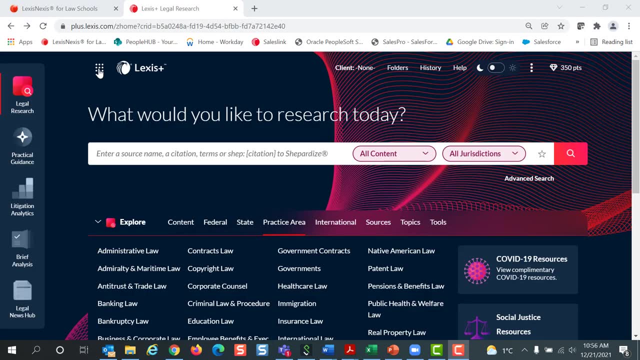 Once you review and confirm this information, you could include relevant information in a letter to a partner or a client. The 50 state surveys are a great place to start your research. Now let's go look at the state law comparison tool. You can access this in one of two ways. 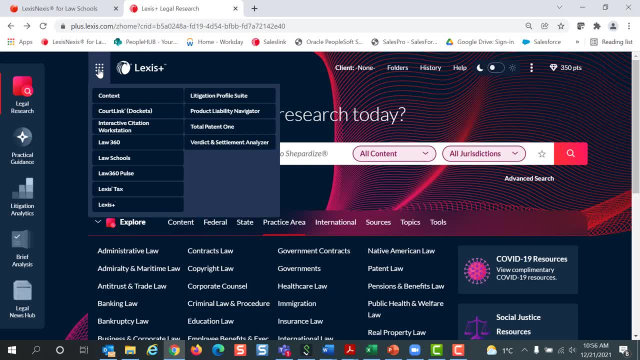 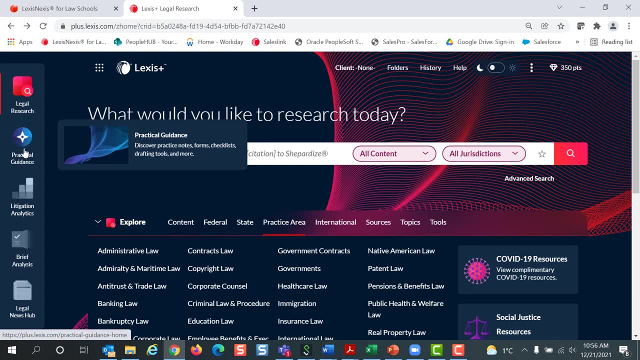 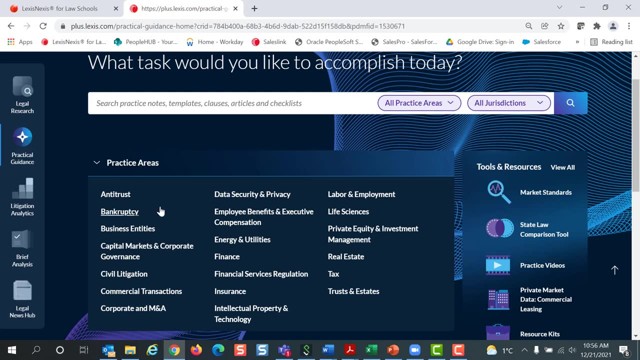 First, you can select the product switcher and select practical guidance from here, or you can access practical guidance in the experience dock on the left hand side. Once you are in practical guidance, you'll notice the standard search box as well as relevant practice areas. On the right hand side, you'll notice the state law comparison tool. 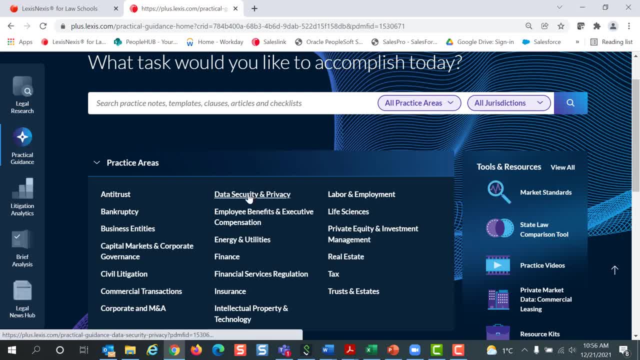 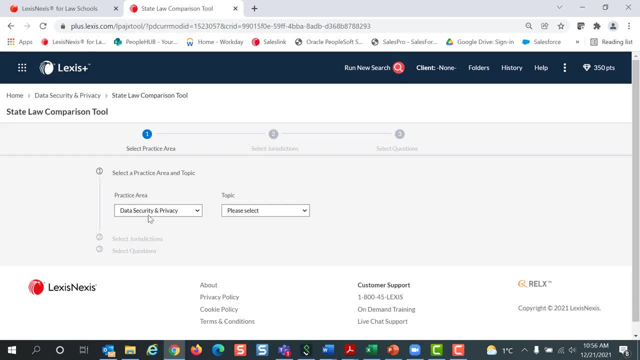 To access this tool, you will first have to select the data security and privacy practice area. Once you've done this, you'll see the state law comparison tool. Uh, a practice area will be saved here. as an option, I'd like to select a topic, so I'll select Data retention and disposal privacy. 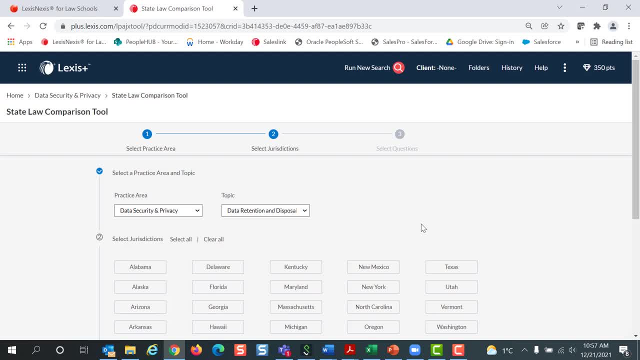 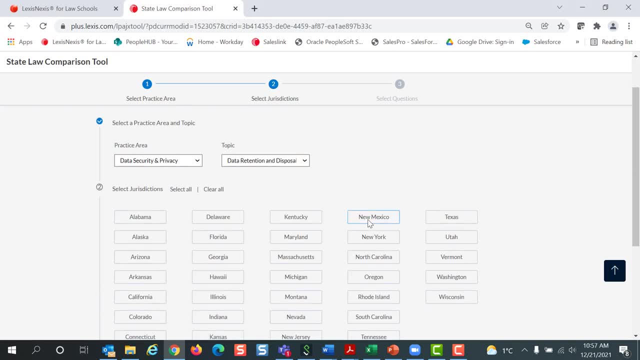 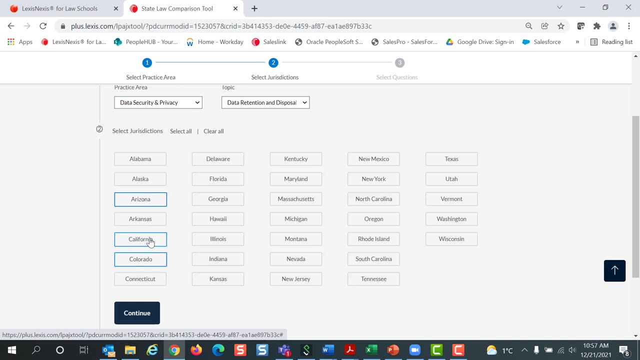 Maybe you've been tasked with determining how long one of your clients must retain records or information and the appropriate way to dispose of them of that information. First, you'll select your jurisdictions. So let's go ahead and select Arizona, Colorado and, why not, let's select California, Once the jurisdictions have been. 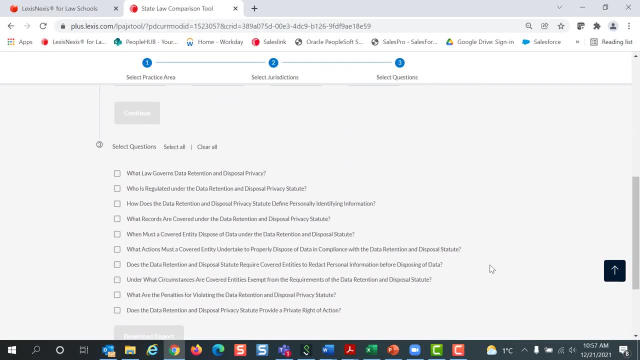 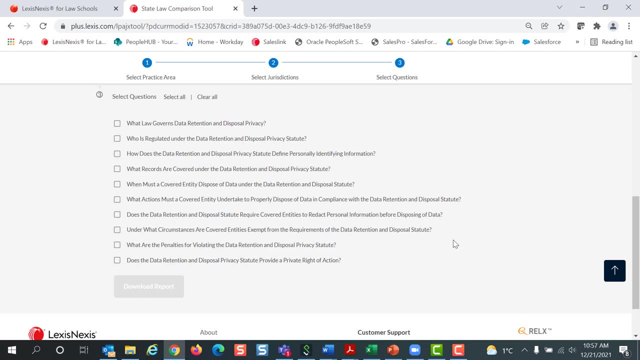 selected, you'll select continue and you'll get a prompt of questions below. These are questions which the system can quickly research for you, So I will select three of them. What records are covered, when must records be properly disposed? and the penalties Once those options have been. 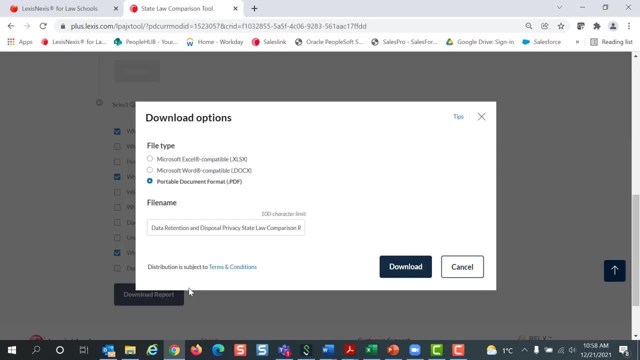 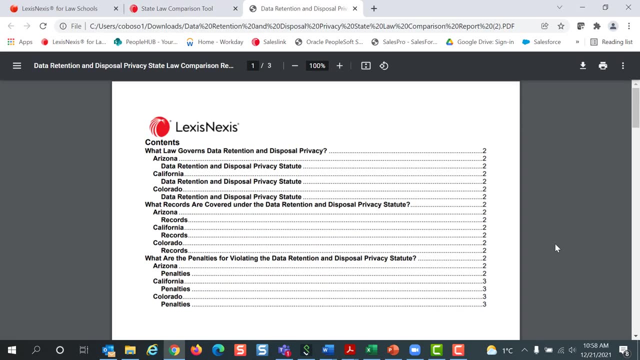 selected, you can download your report. You'll have the option of a file type, and I like PDF, so that's what I will select and we'll download. Once downloaded, you can open that report up and you'll notice. the table of contents organizes your topic and jurisdiction. Now you can review. 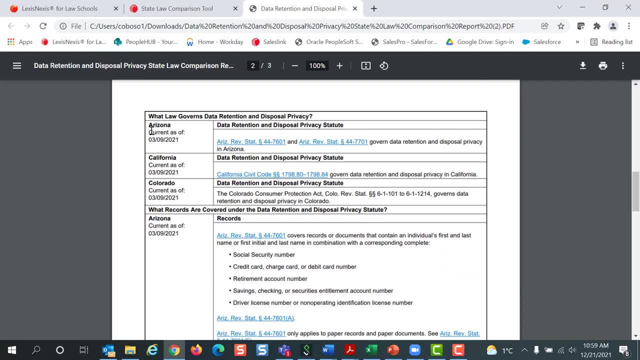 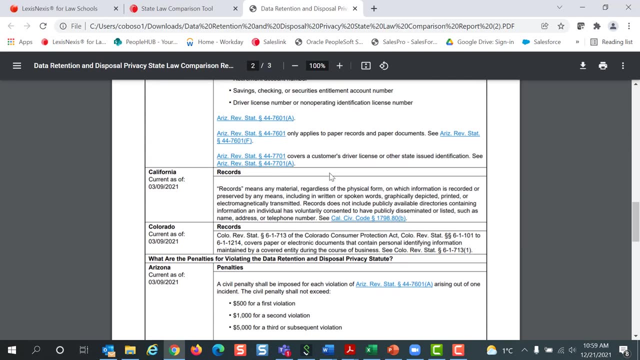 and begin to put the pieces together. This easy to follow chart lets you know that the information is current as of and again. it separates by jurisdictions and includes links to the statutes and other information that you can access from this PDF. Keep in mind that this is also information that you can quickly share with a 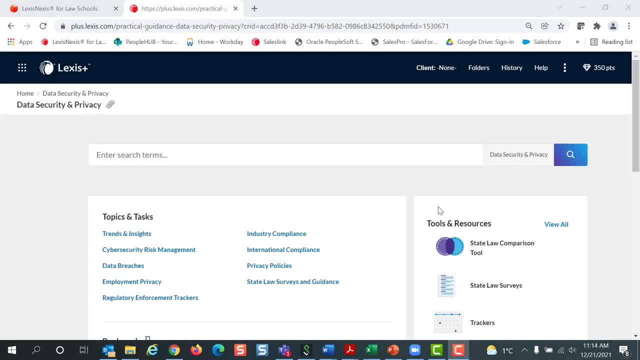 partner or a client in a memo or a letter. Now let's quickly go look at the regulatory enforcement trackers, which can also be found inside practical guidance. Remember, I am in the data security and privacy section under practical guidance. Under the topics and tasks section, you'll notice the regulatory enforcement trackers option. Once you select that, you will. 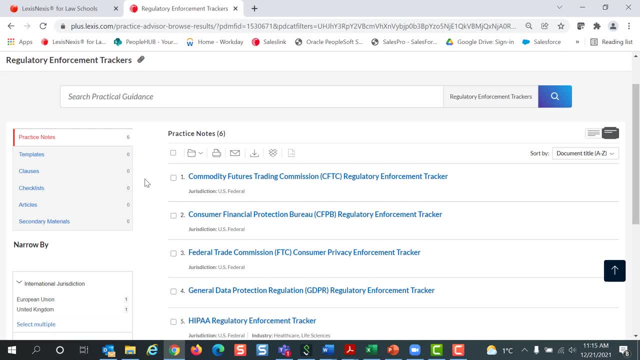 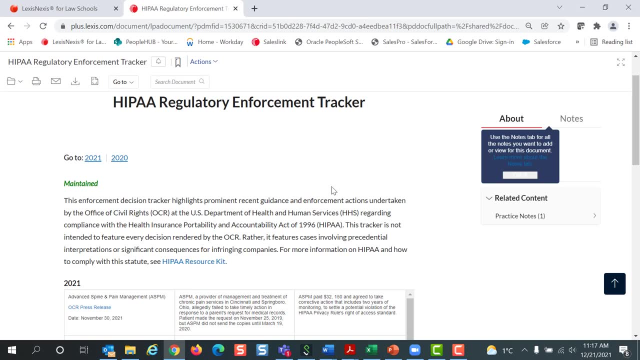 notice the regulatory enforcement trackers on that topic. Here I will select number five. This tracker is not intended to feature every decision rendered by the office of civil rights, but it features cases involving presidential interpretations or significant consequences For companies not following HIPAA. Now, the final thing we'll cover is also in practical guidance. 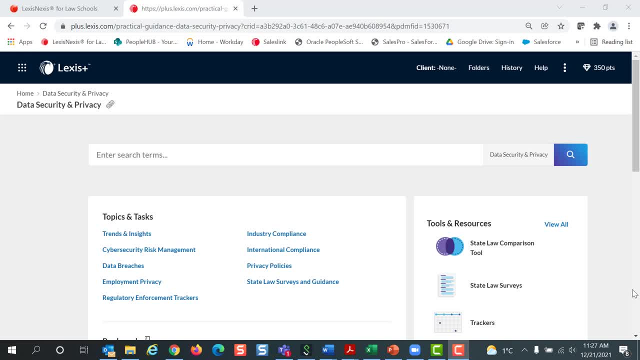 and you guessed it, it is in the data security and privacy section. Here you see topics and tasks that an attorney in this area may deal with on a day-to-day basis. Let's say you've been tasked with drafting a bring-your-own-device policy. I actually had to do this right out of. 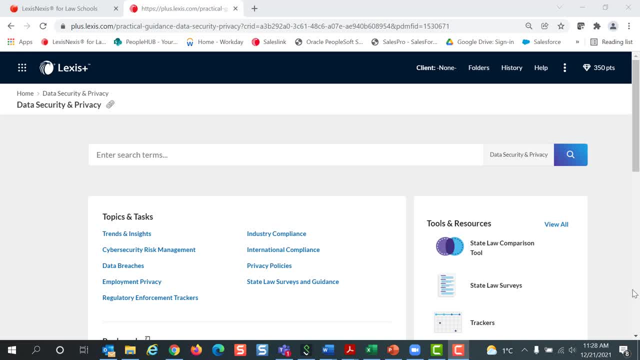 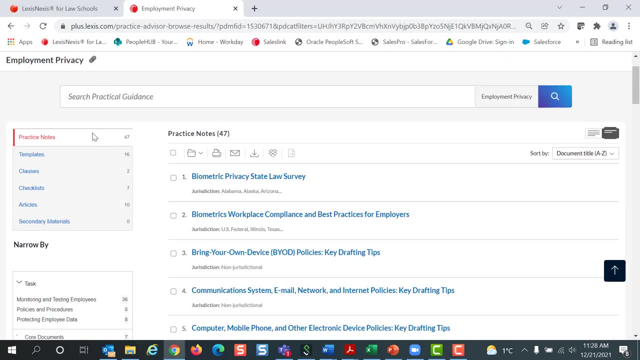 law school. Unfortunately, my firm did not have Lexis, but you do, so I trust that a task like this will be a lot easier for yourself than it was for me. Let's select employment privacy. Once I am in the employment privacy home page, on the left-hand side, you'll notice a set of options: Practice notes. 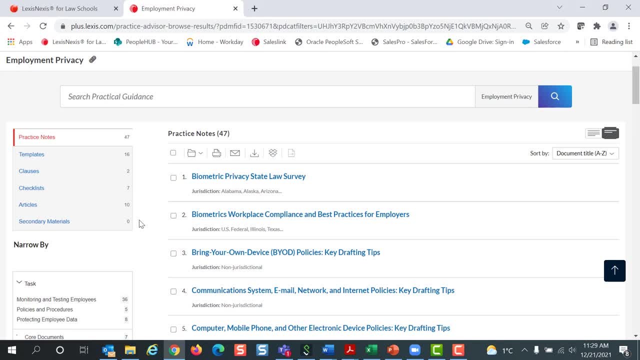 are like encyclopedias on your topic. It is a great way to get a general overview on that specific topic. Templates, on the other hand, will save you a ton of time when trying to draft all sorts of documents you'll encounter in your legal career. If you're interested in learning more about HIPAA and 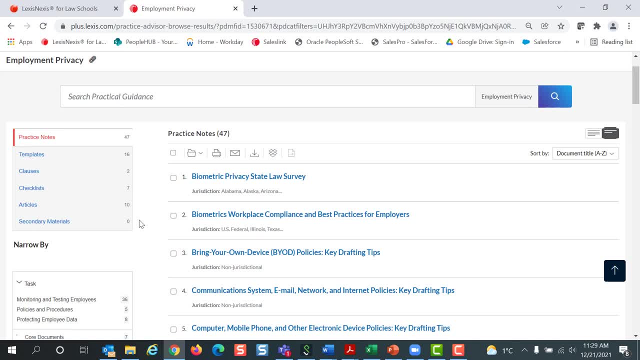 clauses. we'll give you different clauses you can use when modifying your document. And finally, checklists will provide you with a roadmap to make sure you've covered everything on that specific topic. You may also encounter articles or secondary materials that can be useful as you begin your research. So let's go ahead and check templates Once. here you can scroll. 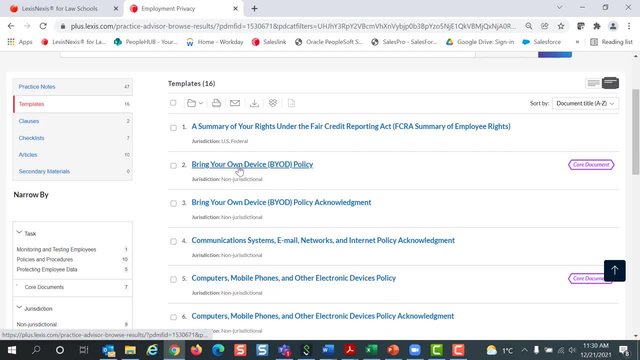 through the options and wouldn't you know? option number two is a bring your own device policy. Now let me direct your attention to the right hand side. anytime you see the core document on an option, this is the system telling you that this is the most important document on this subject. so